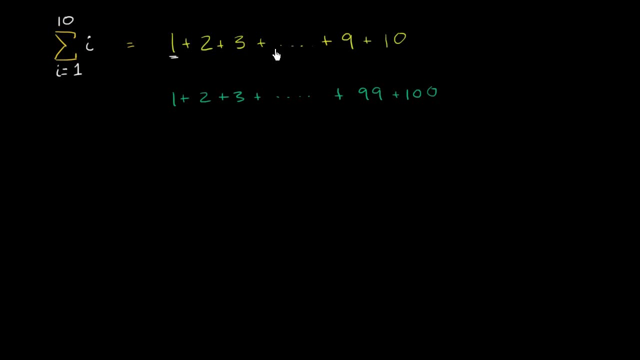 i is 2.. Put the 2 down And you're summing each of these terms as you go, And you go all the way until i is equal to 10.. All the way until i is equal to 10.. So, given what I just told you, I encourage. 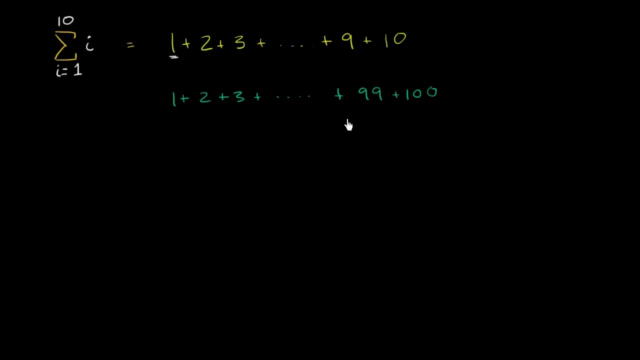 you to pause this video and write the sigma notation for this sum. I'm assuming you've given a go at it. Well, this would be the sum, The first term. well, it might be easy to just say: we'll start at i equals 1 again. 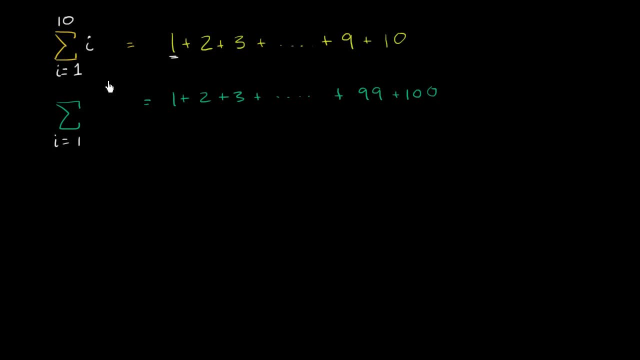 i equals 1.. But now we're not going to stop until i equals 100.. And we're going to sum up all of the i's. Let's do another example. Let's imagine the sum. Let's imagine the sum from i to 10.. 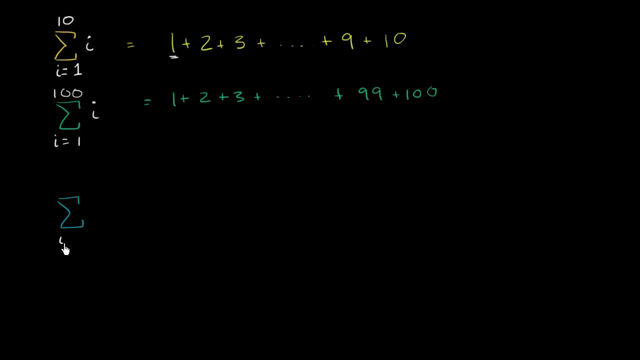 Let me do this From i to 10.. From i equals 0 to 50 of I don't know. let me say: pi i squared, Pi i squared. What would this sum look like? And once again, I encourage you to pause the video and write it out. 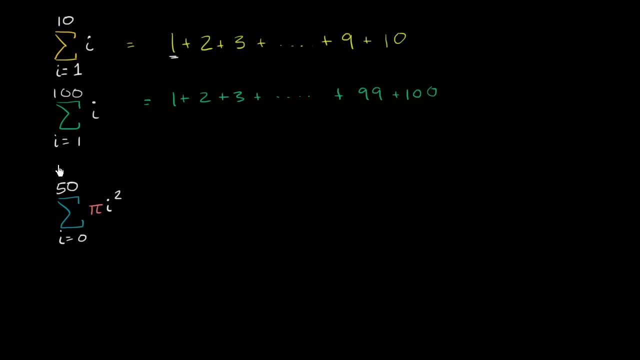 I kind of expand out this sum. Well, let's just go step by step. When i equals 0,, this will be pi times 0 squared, And that's clearly 0.. But I'll write it out: Pi times 0 squared. 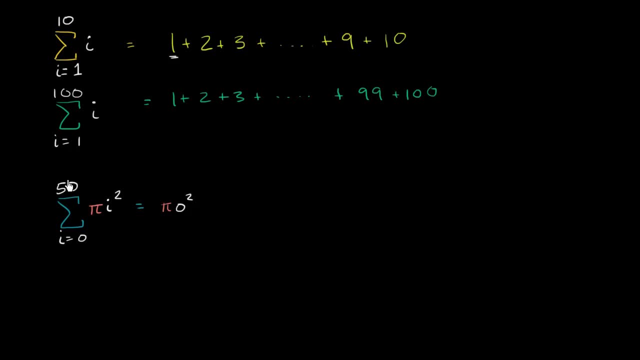 Then we increase our i And we make sure that we haven't hit this, that our i isn't already this top boundary right over here, or this top value. So now we said i equals 1. Pi times 1 squared. So plus pi times 1 squared. 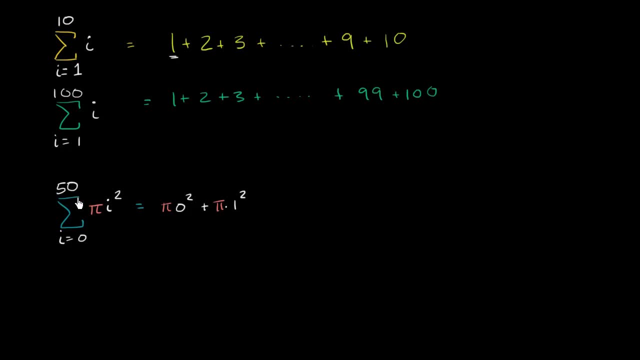 Well, is 1 our top value right over here where we stop? No, So we keep going. So then we go. i equals 2. Pi times 2 squared, So plus pi times 2 squared. I think you see the pattern here. 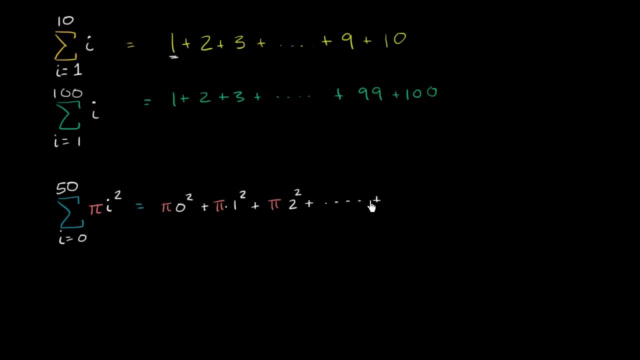 And we're just going to keep going all the way until at some point. we're going to keep incrementing our i. i is going to be 49.. So it's going to be pi times 49 squared, And then, finally, we increment i.